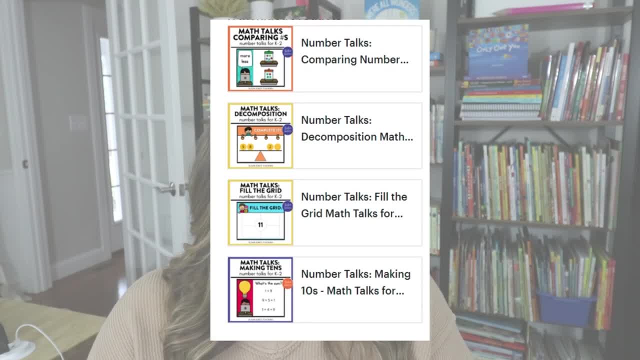 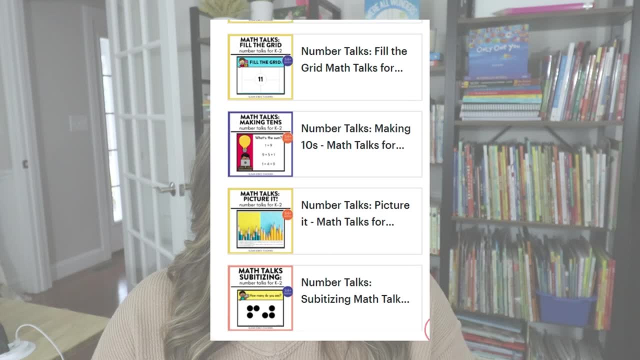 different types of math talks I love doing in the classroom. So here students can work on subitizing, they can work on comparing numbers, they can discuss which number or object doesn't belong and why. they can play fill the grid where they figure out different ways to make a number. 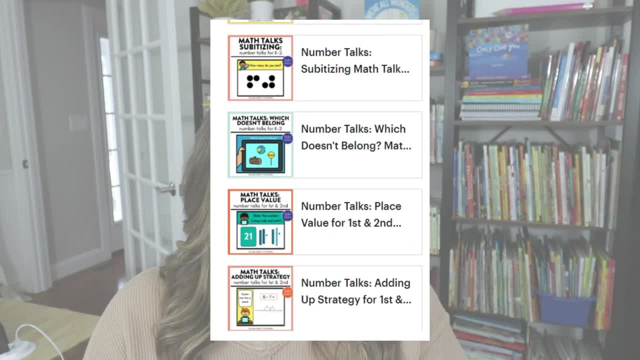 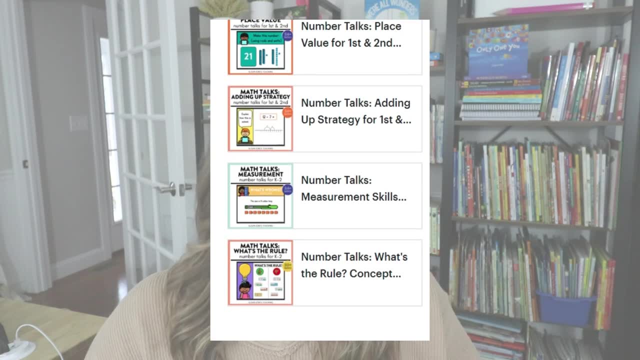 we focus on the strategy making tens decomposition. I have picture prompts, place value slides to focus on. I have math talks for the adding up strategy as well as specific measurement ones, and a what's the rule math talk bundle where students will look at concept attainment and they have to decide what the rule is. 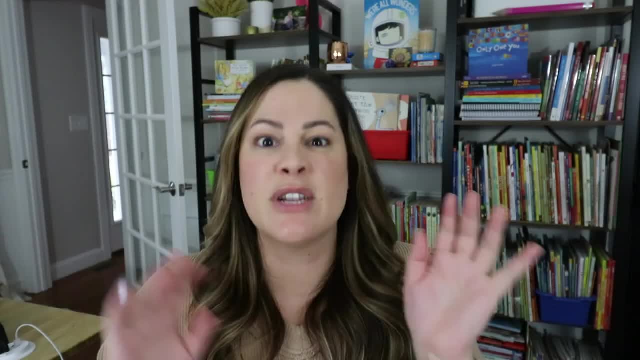 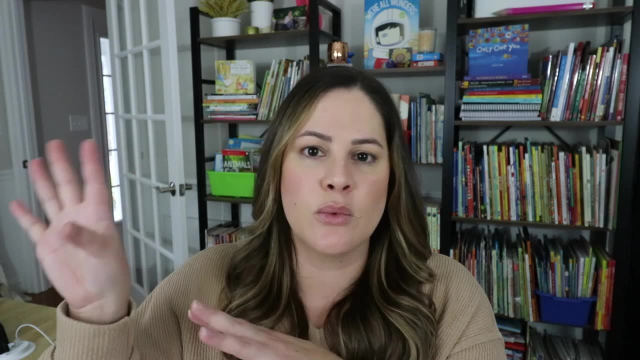 and why it isn't applied on the thumbs down side. So, as you can see, I've compiled a bunch of those in a big bundle. I also sell each of the different strategies and skills that you can work on separately for like two dollars each. so if you 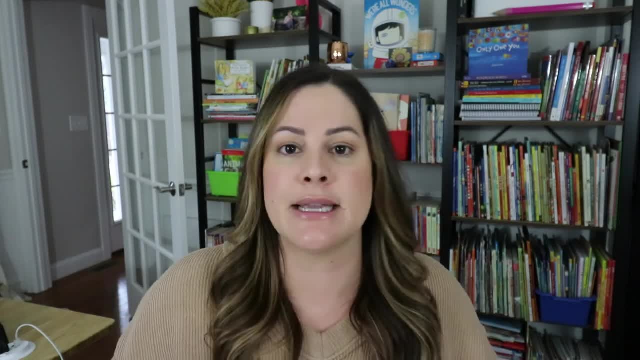 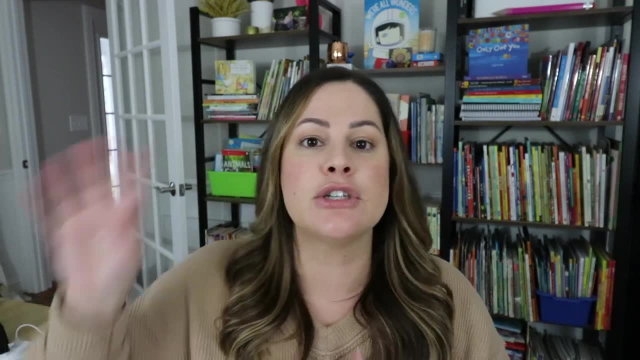 just want some number talk, you can do that. If you want to learn more about math talk, you can go to numbertalkscom for the adding up strategy, for example with subtraction. then you could just get the adding up strategy. or if you just want the subitizing number talks, you could also grab those. 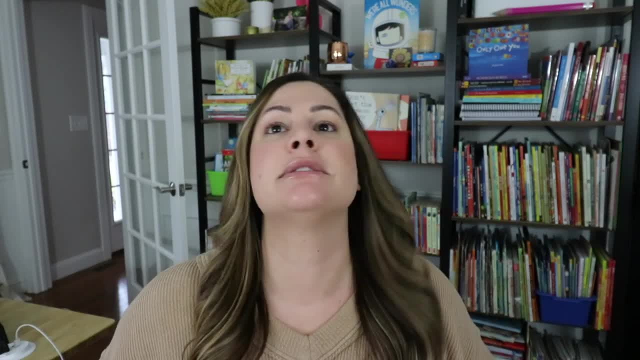 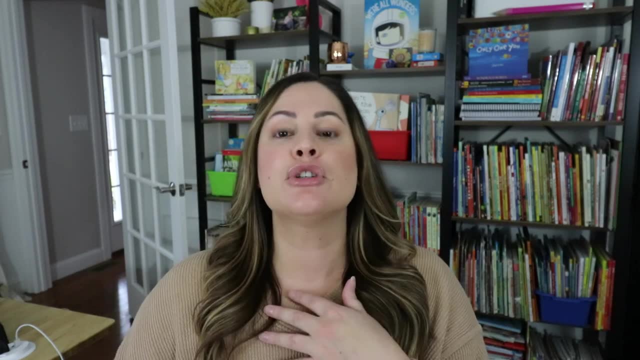 as well. So you can see that you can have a math talk really around any math skill that you want to deepen your students conceptual knowledge around. So, all that being said, what is a number string? Now, a number string is a type of math talk that I've seen numerous times before. I. 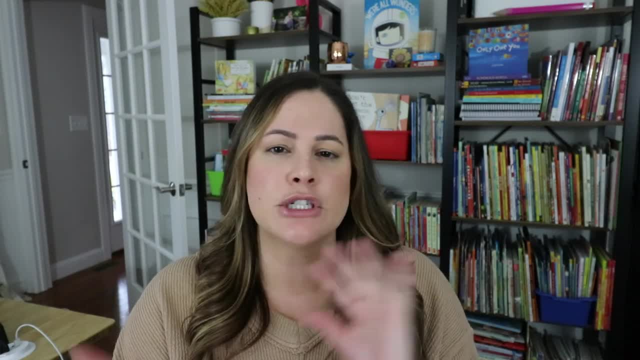 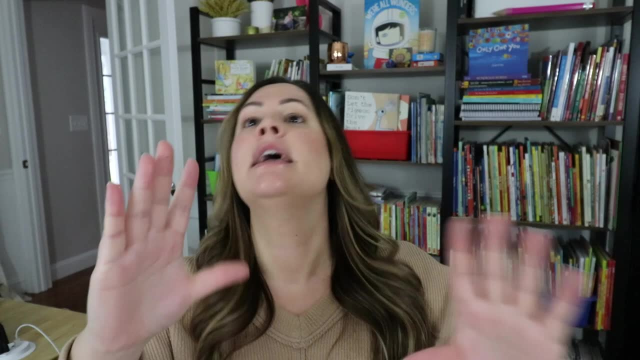 believe Sherry Parrish has an entire book with number strings. she calls them number talks but technically they are number strings. So a number string is when you have a set of related problems and students go through the problems, usually one at a time, and they try to identify. 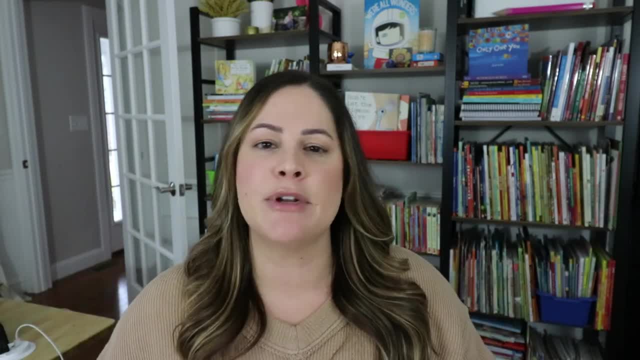 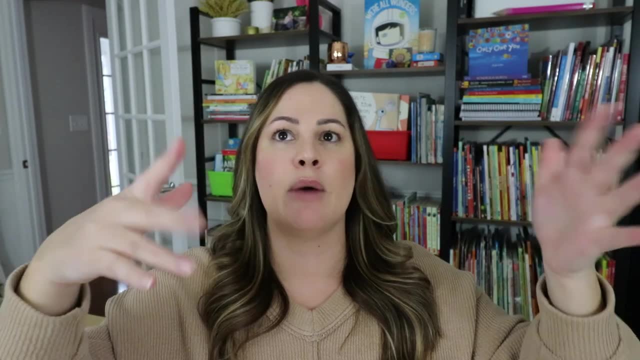 the relationship between the problems And they're kind of set up in a specific way, with a helper problem or like a base problem, and then it goes into something that would illustrate the strategy you're working with And then students go back to the base problem and then use the problem. 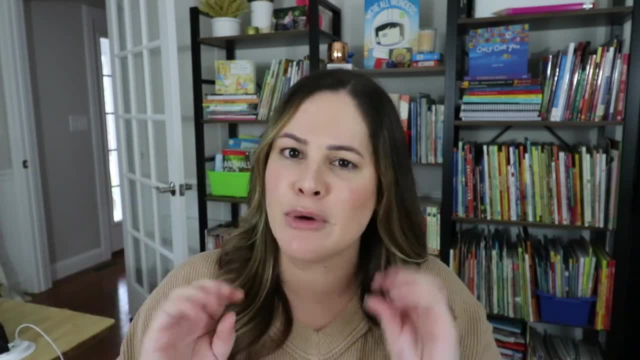 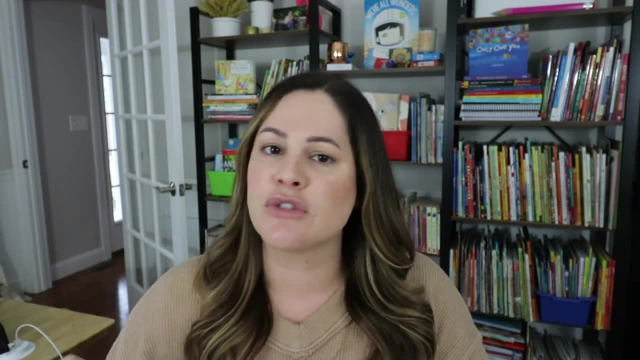 to work on the strategy. Now, that sounds pretty abstract. don't worry, I'm going to show you plenty of examples so you know how to do this. Now, just to point out before I do go into a few examples, so you can see what number strings 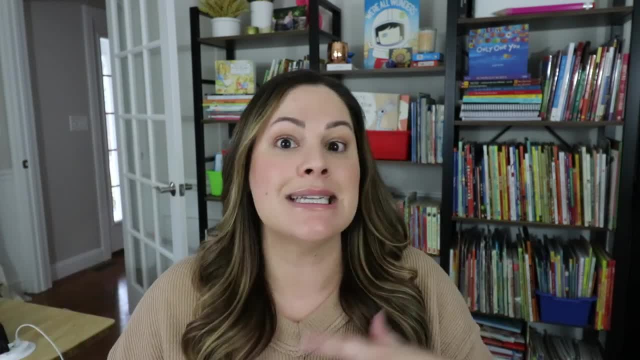 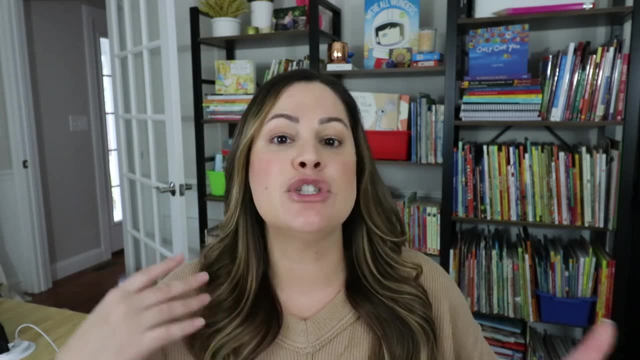 really are and how they work with your students. I do want to emphasize that this is a type of math talk, So a lot of the math talk norms you'll have with your students are going to remain the same. This means you'll want to try to keep these student-led, So you are showing them problems. 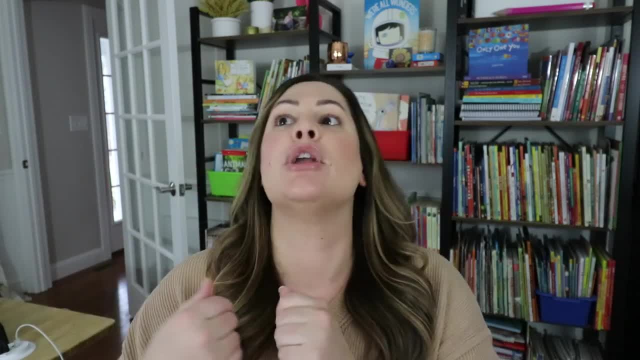 on the board and you're kind of guiding them towards an answer, but you are not explicitly teaching them the answer just yet, right? So you're kind of guiding them towards an answer, but you are not explicitly teaching them the answer just yet, right? 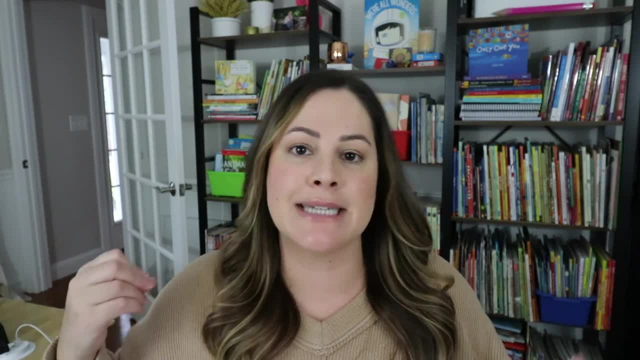 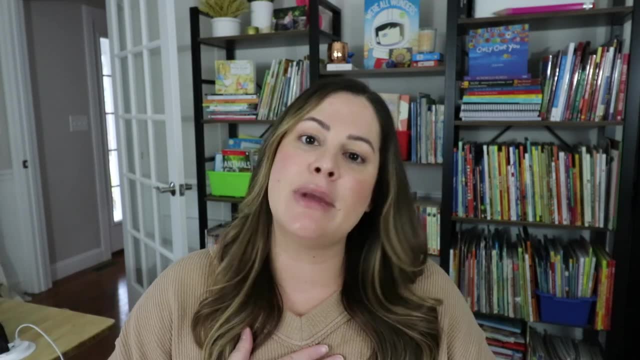 We still want them to talk around the ideas. We want to write down and record the ideas. But a few things are different about a number string. First, it's going to be a little bit longer than my typical math talks. I know plenty of other people have math talks where they talk. 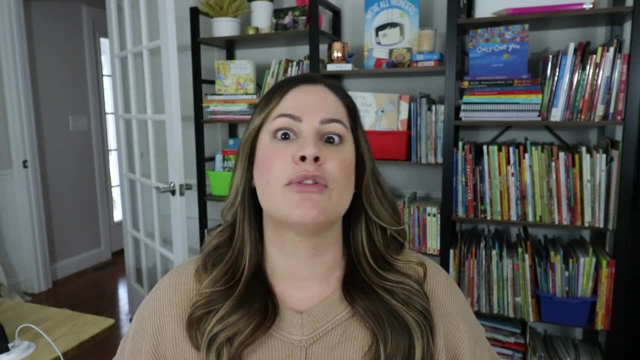 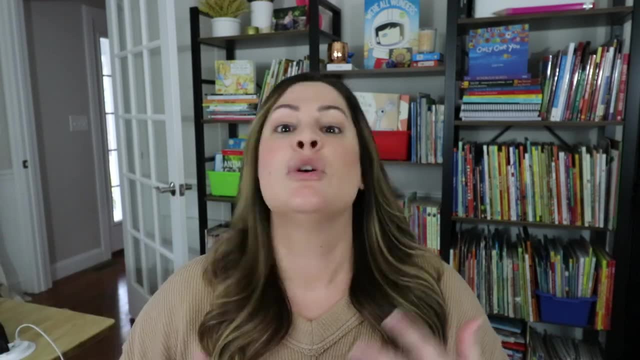 15-20 minutes during the math block time In K-2, I find it hard to hold their attention for that long And I find that if we just do it every single day for about five minutes, we still get, you know, really great students that are able to talk about math. But since number strings are set, 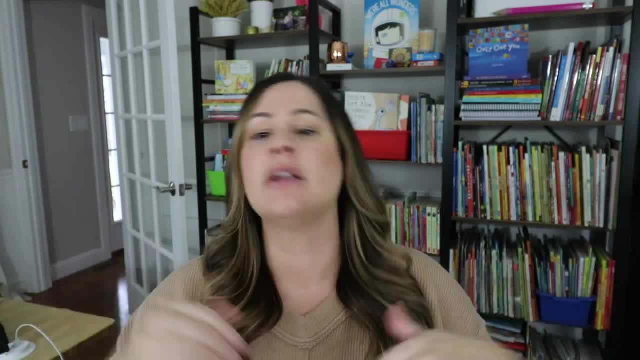 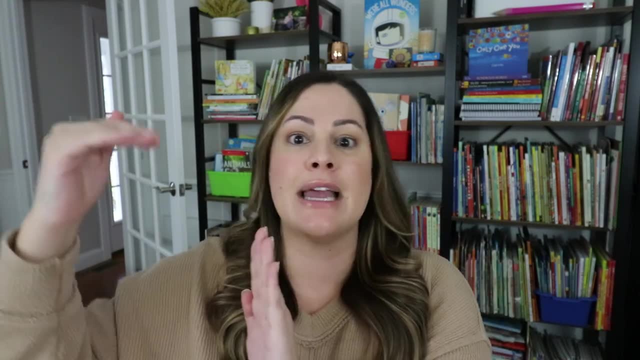 up as not one particular problem, that you're talking all about and discussing all the different ways you can solve this one problem and how we know the answers. instead, again, it's set up as a set of problems. Maybe there's four problems, maybe there's five, maybe there's six, And you 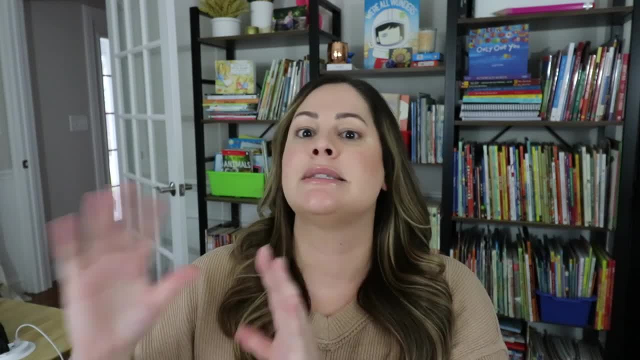 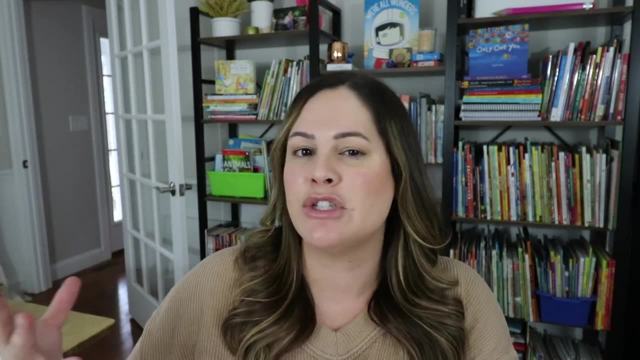 want to talk about the relationship between them. We don't instead go super deep on one. we go deep on all of the problems together, So these would take about 10 minutes to go through. All that being said, let me just dive into an example of a number string. 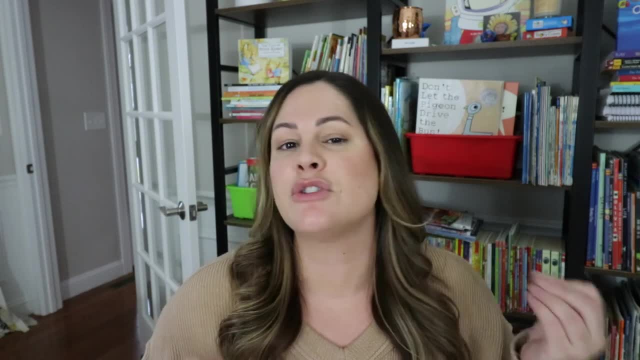 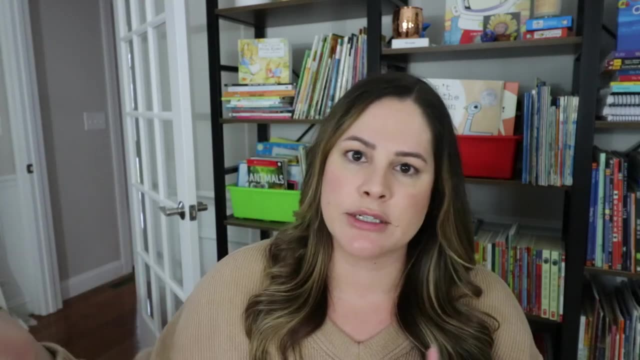 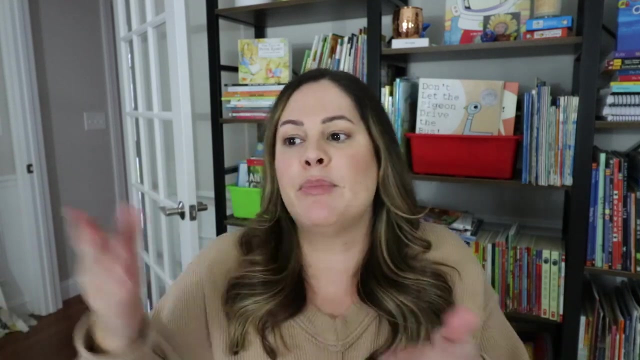 Now, number strings are great to use when you're trying to illustrate a strategy that might be a little abstract for students. For example, in first grade, if you were teaching students the doubles plus one strategy, you can easily tell your students: okay, three plus three, we know, is six, right, They've memorized that. So three plus four must. 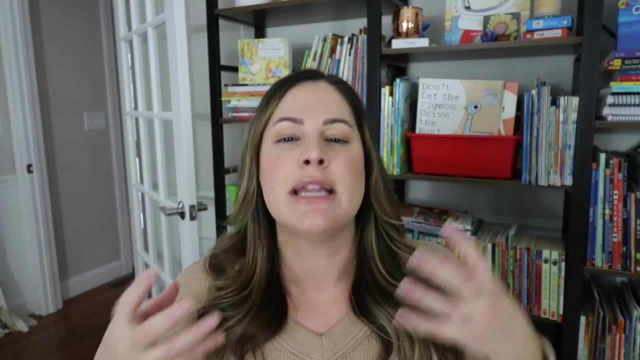 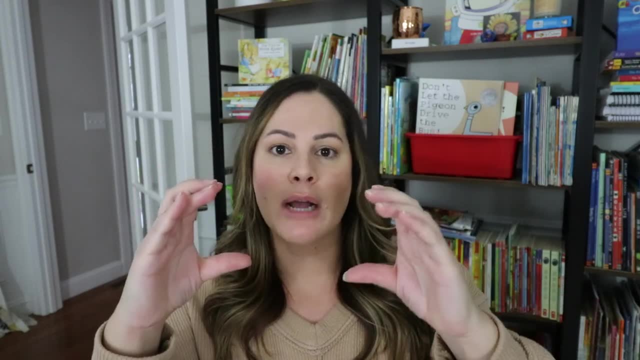 equal one more seven. You can tell them this, but hearing all those numbers over and over again is pretty abstract. We want to show them visuals and we want to show them helper problems to help them understand this concept. So let me show you. This is exactly how I would start off. 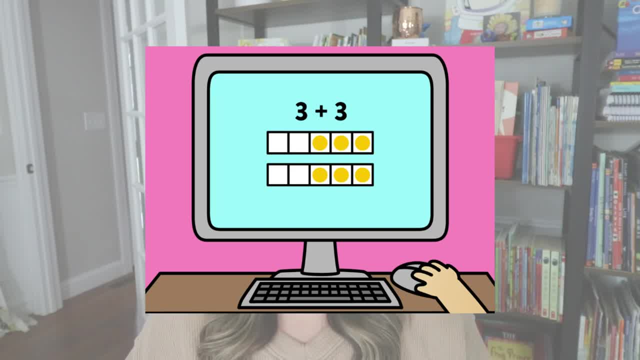 a number string with my students Now. since I'm teaching doubles plus one at this point, I would obviously expect my students to know their doubles facts, So I would simply show them here. three plus three is what? And we have a visual here. We have the three and the three in five. 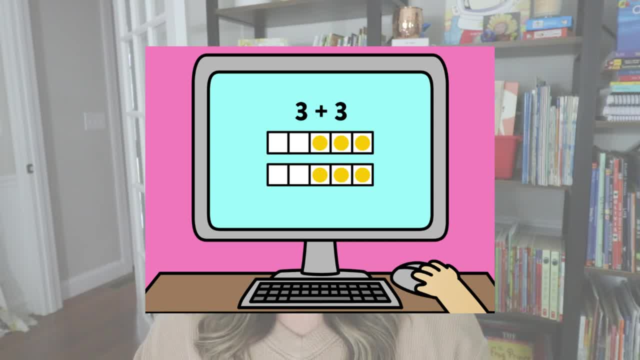 frames and they would tell me it is six. Now I could ask them a little bit more. I'd ask them: how did you know? Do we agree? Do we disagree? Okay, But again, we are not spending a lot of. 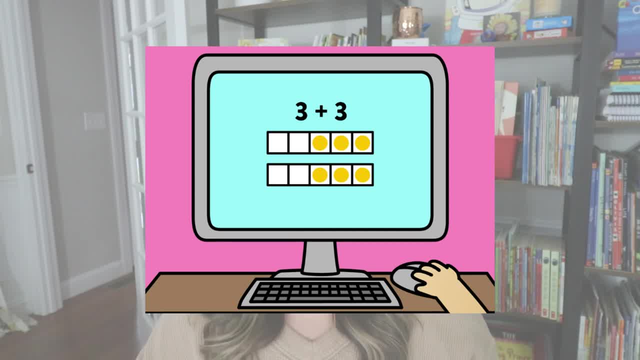 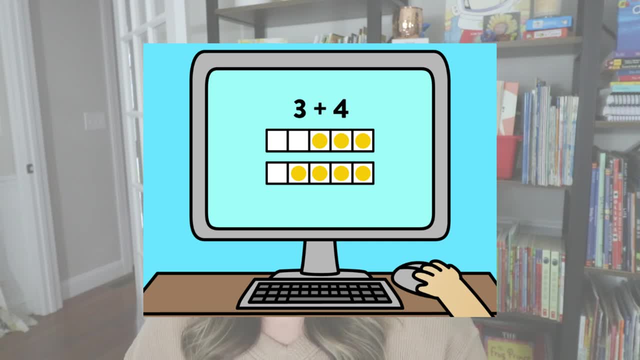 the entire five minutes on this one slide. We're spending 10 minutes going over 10 slides. Then I would go to this slide. Okay, Three plus four. So I would again ask my students how they solved it, And if nobody points out that we already knew three plus three, I could go back. 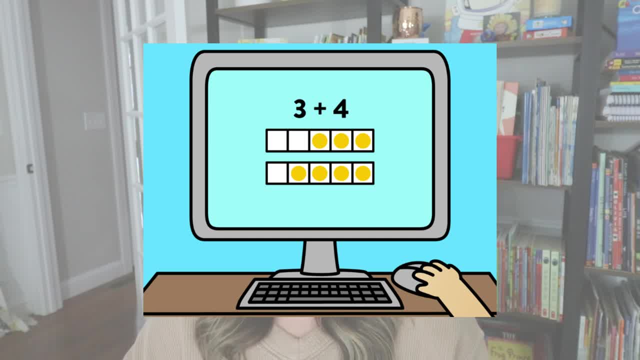 to the other slide and ask my students: what do I notice about these two problems? here We have three plus three and three plus four. Look at the visuals. I might get up there and I might even circle. three plus three and three plus four. Look at the visuals, I might get up there and I might even circle. 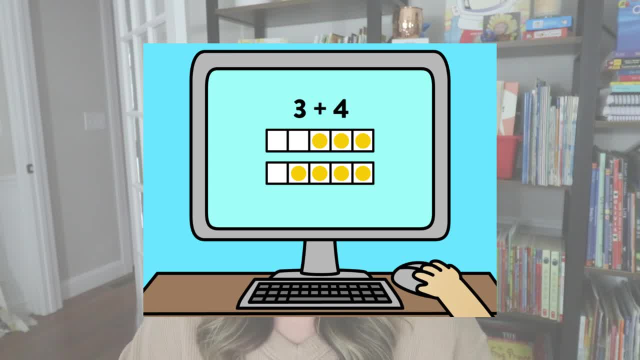 look at the visuals. I might get up there and I might even circle the top three and circle three on the bottom And notice how it's the three, the three plus the one equals seven. I could record that as three plus three plus one equals seven, And then I could. 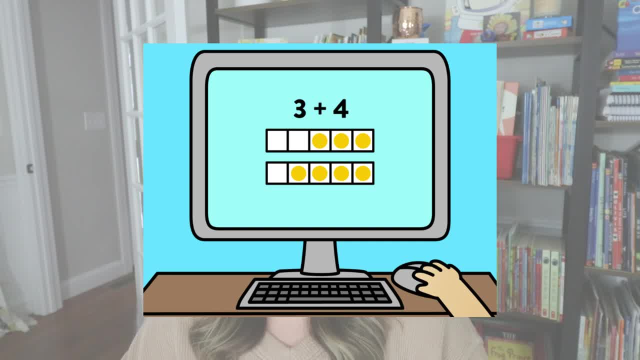 also shorten that into six plus one equals seven, because we already know that doubles fact of three plus three. So you can see that this slide is the one we're going to spend a little bit longer on, since we are going into depth about this doubles plus one strategy. Then I show the next slide. 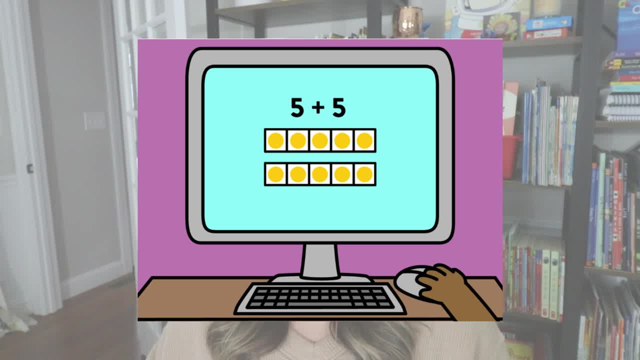 five plus five Now. notice that this slide is the one we're going to spend a little bit longer on. since we are going into depth about this doubles plus one strategy, Then I show the next slide: five plus five Now. notice I didn't go into another doubles plus one yet. This is in your. 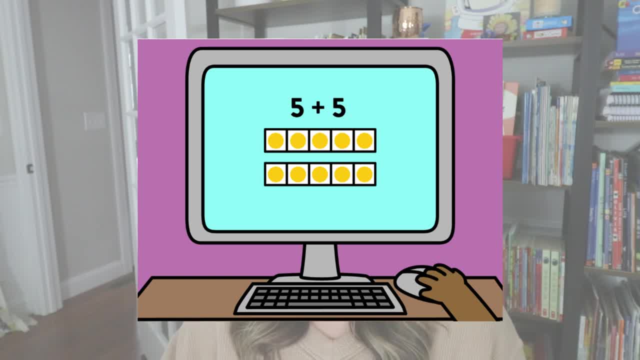 number string. You want to make sure that you have these base problems or these helper problems to get students to go back to what they know, and then we will make it a little more difficult. So we already know this. Five plus five is a doubles fact. What is it? everybody Ten. 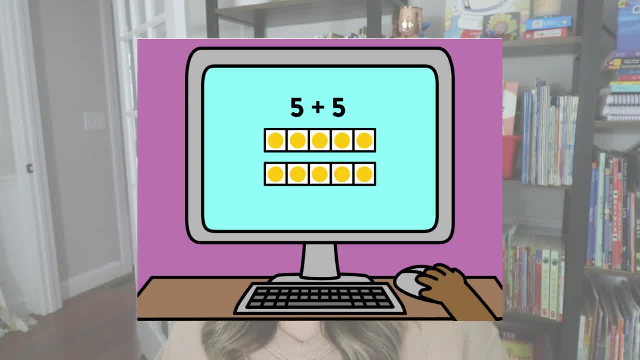 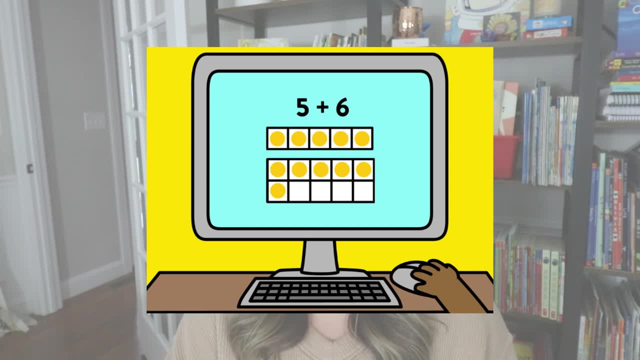 Okay, Well, as five plus five equals ten, what is five plus six? Take a look at this one Again after we've gone through the three plus four. they might say: okay, well wait, we already know. five plus five equals ten. What is five plus six? Take a look at this one Again after we've gone through the three plus four. they might say: okay, well wait, we already know. five plus five equals ten. 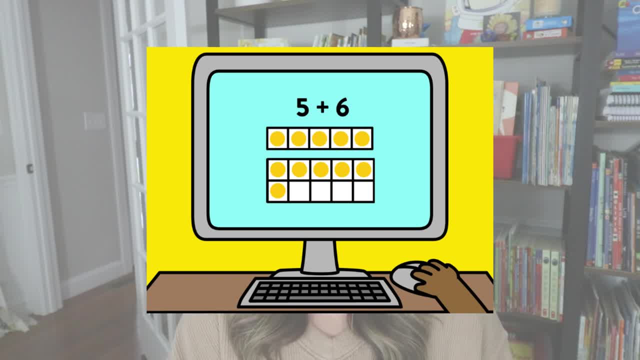 And again on the board. I can circle those fives right away. Plus one more equals eleven For this type of skill. I would continue using visuals a few more times, and then my last couple slides will always be more abstract when my students are ready for it. If we get to an 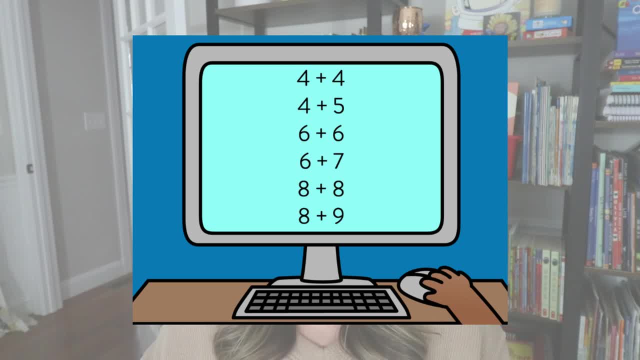 abstract slide like this one where I just have a bunch of equations and my students are floundering or they really don't get it. yet we take a step back. We practice more with visuals, But we do like to get to this abstract portion. Four plus four: what does it equal? everyone Ten. 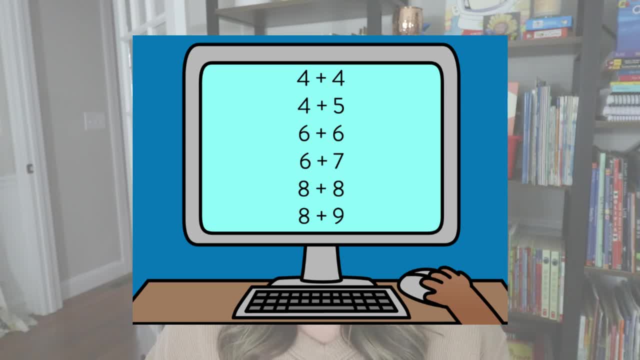 Eight. So if four plus four equals eight, then four plus five must equal nine. Back to a helper problem. Six plus six, what does that equal Twelve? Then six plus seven must equal thirteen. Back to our helper problem. Eight plus eight, what does that equal? Eight plus nine? 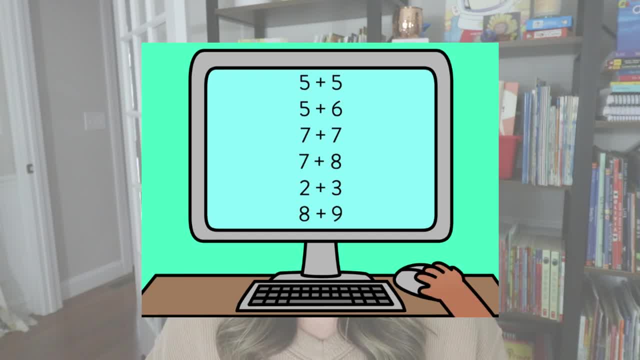 So you can see here how this type of number string would work. And then, lastly, I do like to include one more of these Here. I have two helper problems with the five plus five and the seven plus seven, but my last two I don't have a helper problem, I just. 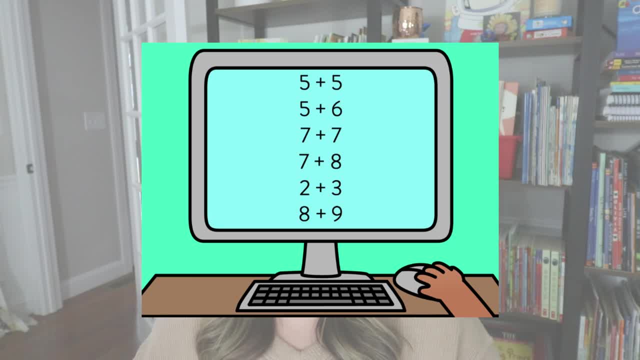 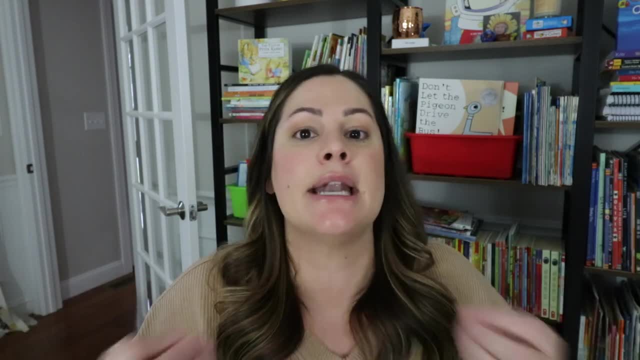 see if they can try to solve it with the doubles plus one strategy without going back to the helper. So those six slides that I just went over with you are part of a ten slide number string math talk that I would have with my students. Now, for time purposes I took out four more slides that just 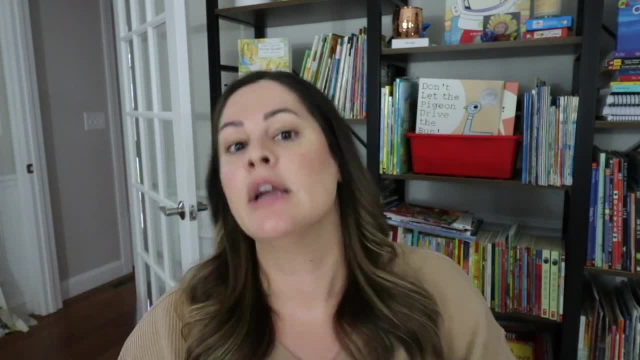 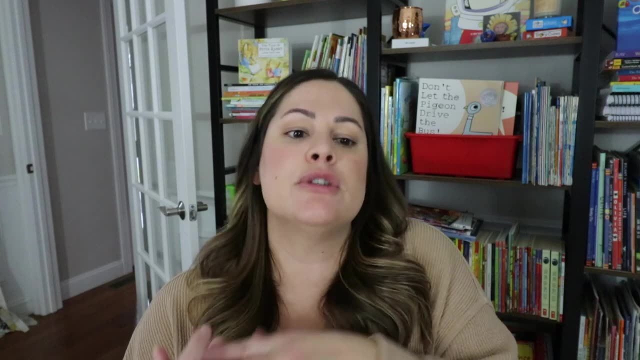 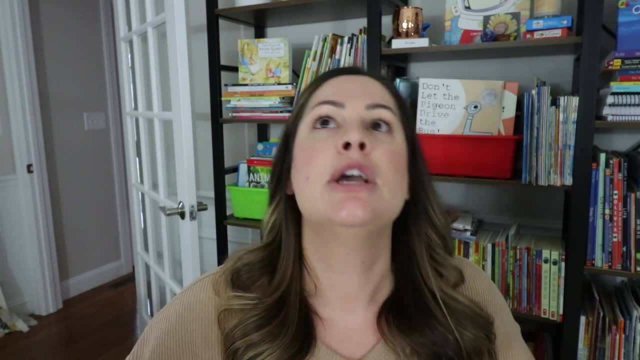 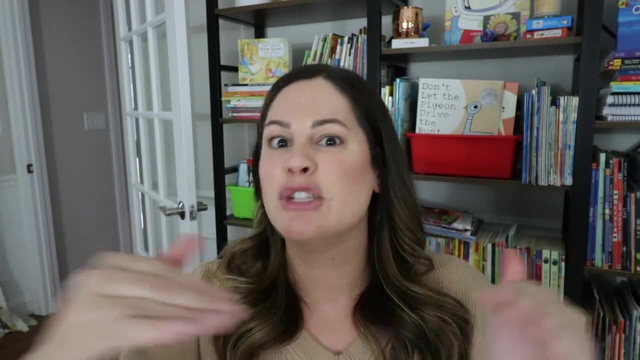 and do that. I'm going to go ahead and do that. I'm going to go ahead and practice that doubles plus one strategy. without it being so abstract at first, We do of course, move there, So that's why we have our number talk with visuals first, and then we try to get to that. 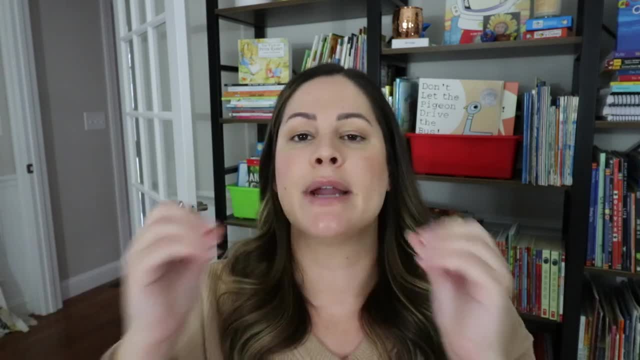 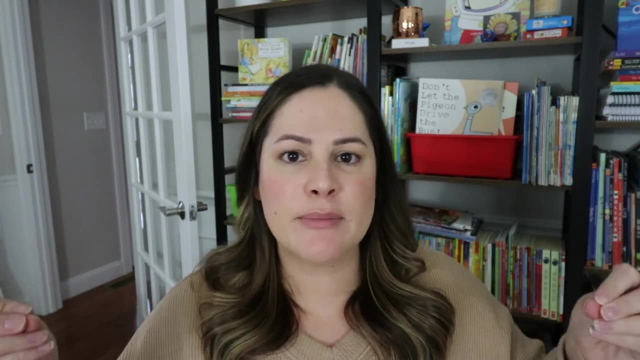 abstract point. But along the way students are able to break apart those numbers. They're able to see how they relate to the actual doubles before practicing it themselves. So there you have the outline of a number string, right How we want to go ahead and set them up to help our 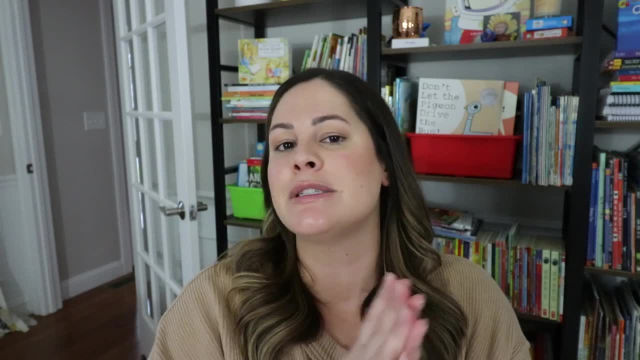 students discover these new strategies. And now that you understand the setup, let's go ahead and get started. So let's go ahead and go ahead and set them up to help our students discover these new strategies. And now that you understand the setup, let's go ahead and go ahead and 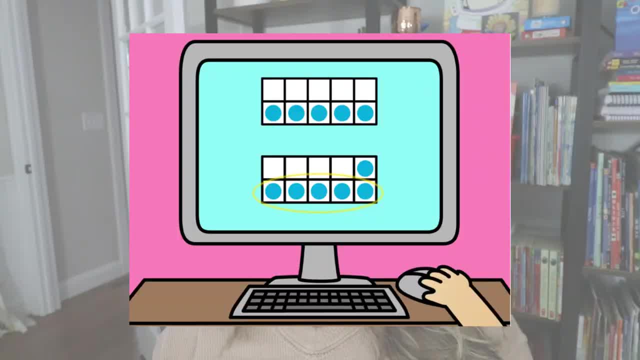 let me show you a few more examples of ways you can use number strings. I also love to use number strings in kindergarten and first grade when we are trying to teach them to anchor a number. I want my students to anchor the number five, for example, in this example, So I will have a five. 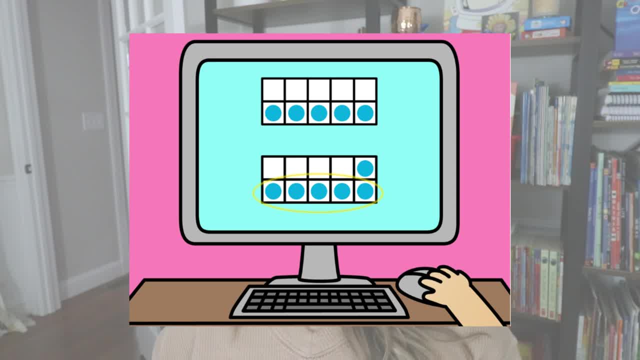 up at the top and I'll ask students just to tell me: what number do they see, how do they know, et cetera. And then they'll say, oh, we have five dots, It fills in, you know, half the 10 frame. 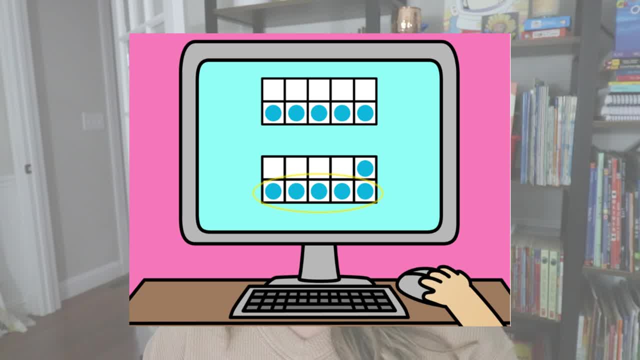 That's the number five. And then, once we get there, I'll say, okay, now look at the bottom number, What number is that? And they'll know that it is six And I'll ask: how did you know? Now, I thought. 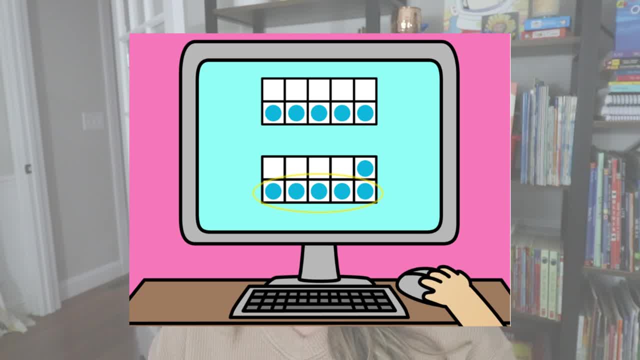 about kindergarteners while I was doing this slide. So here I also have a glowing oval over the bottom five. So of course they can tell me that you know they counted up each dot individually. Um, but I'm trying to guide them towards the fact that six is just five and one. 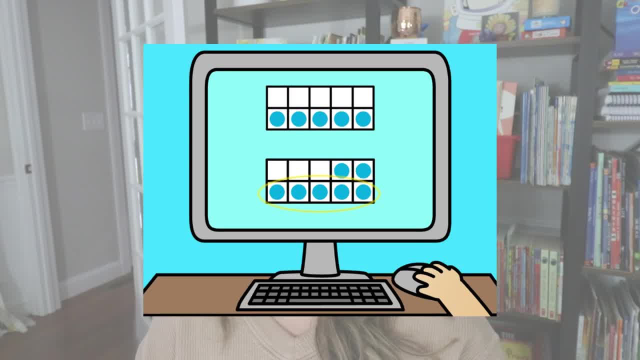 more. Then we go to the next slide. I'll ask my students again: what number do we see up at the top Five And what number do we see at the bottom Seven? How did you know After going through the first slide- hopefully we'll quickly get to- seven is five and two more. On the third slide we 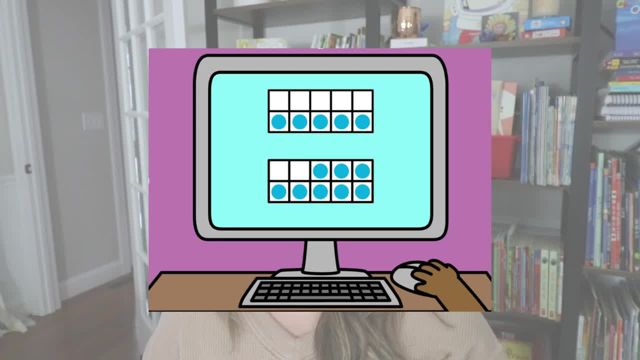 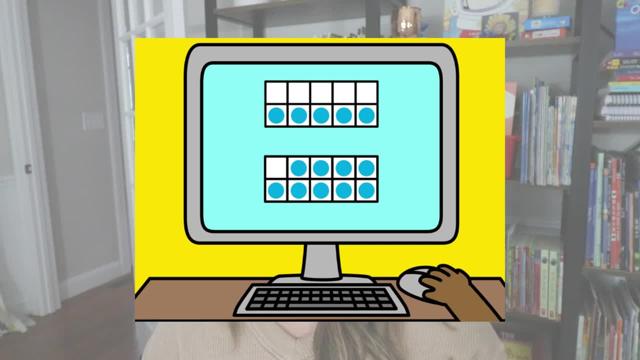 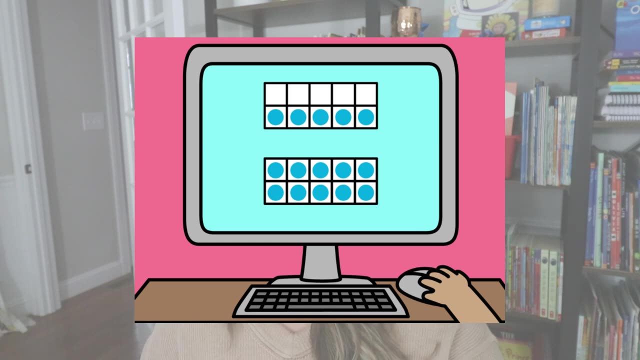 continue with five and eight, but here I took away that scaffold, I took away the glowing oval to show that you know, eight is five plus three more. The next slide is the number nine And the last slide is the number 10.. So once we've gone through those relatively quickly, remember this is all in one. 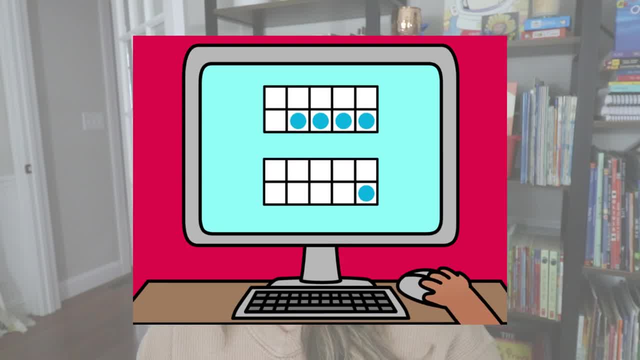 math talk, Then I will show my students this slide right here. Hmm, What number is shown between both of these 10 frames? What number do we see up at the top Nine And what number do we see up at the bottom Ten? And I want my students to recognize that four plus the one more equals five, And I 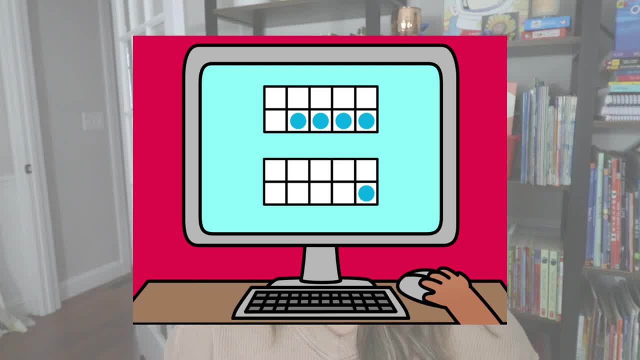 want them to visualize the fact that they can take this little dot from the bottom and they can move it up in their head to know that that five there, when we have half of a 10 frame completed, it's five. So, as you can see, some of the previous slides would probably go a little quicker. 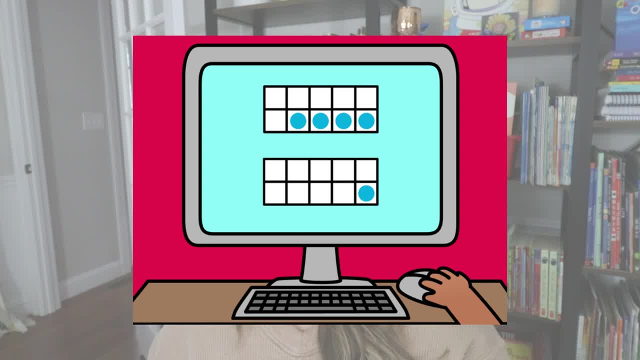 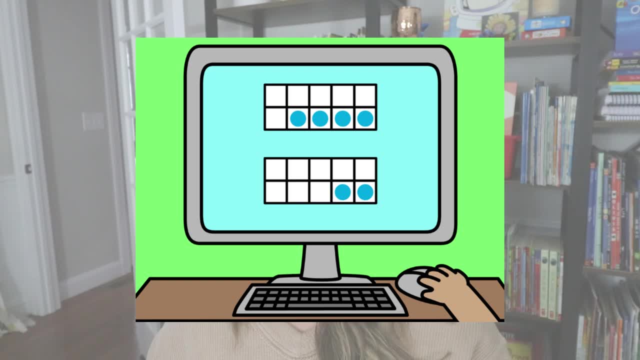 and then we get to something new and we're like: hmm, how can we think about this? Again, this is a math talk. Then we go to the next slide. Well, if the last one was four and one equals five, what's four and two? Again, I want them to visualize. They can take one of those circles. 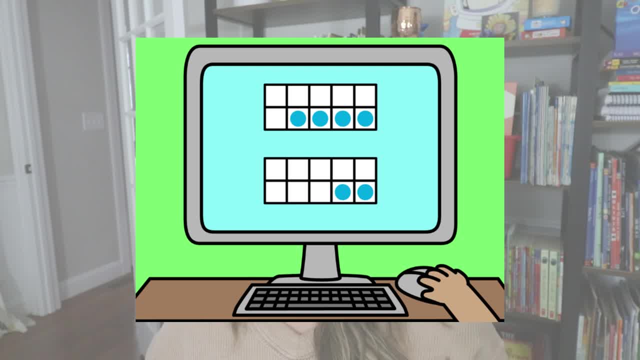 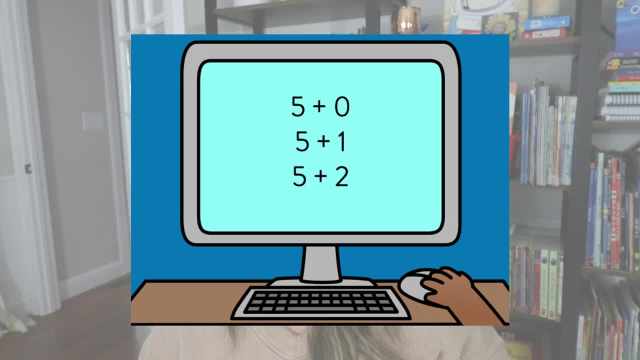 complete the five frame up there, and then they have five and one more is six, And then similar again is four and three, And then we go into our abstract portion. We have five plus zero, five What's five and one more Six, What's five and two more Seven. And what I'd be looking for when 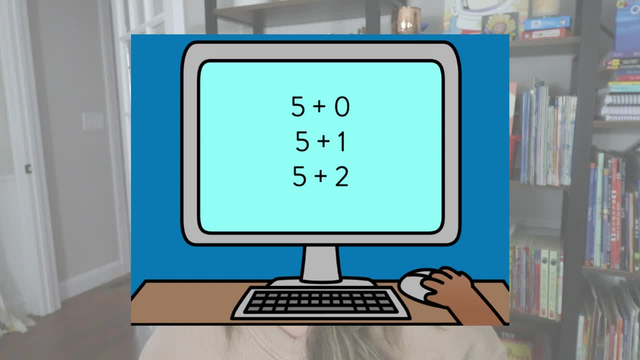 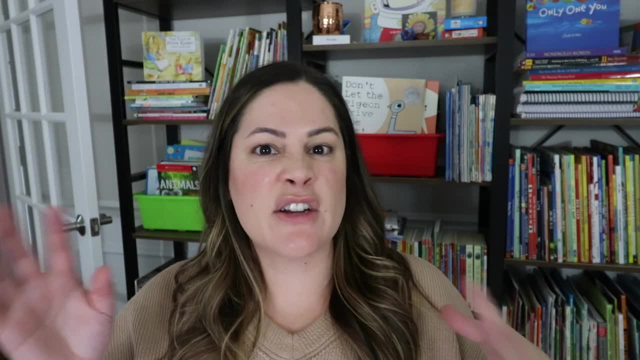 students are solving this is for them to count on from five. I don't want them using individual manipulatives just yet. I want them to be able to count on from five. I want them to be able to do it because, again, we're working on five being that anchor number. I also created a very similar 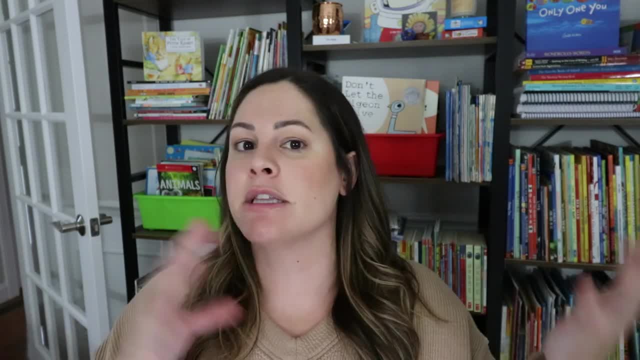 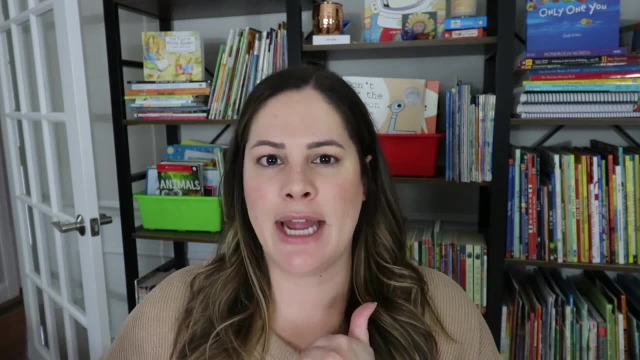 number string of 10 slides to do that same thing, but instead of anchoring the number five, we are anchoring the number 10, specifically thinking of those teen numbers. So it's set up in a very similar way. Now I want to zoom through one more strategy, just to show you another example of these. 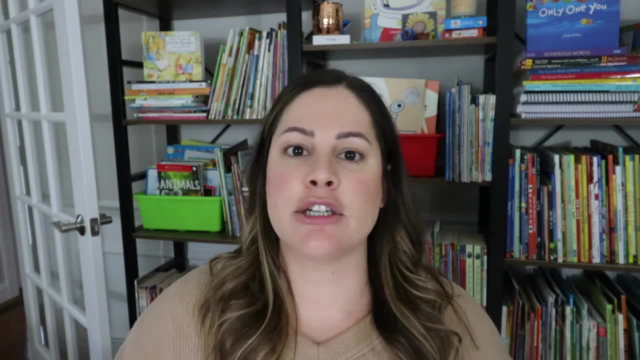 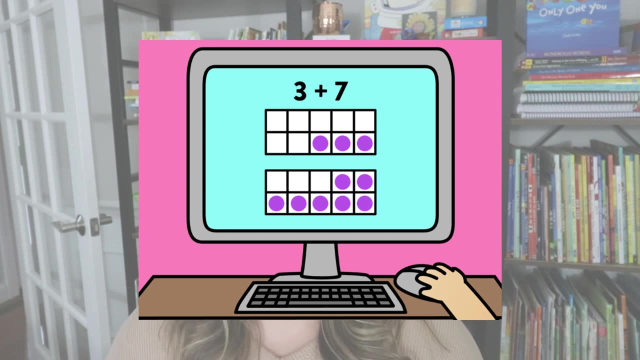 number strings, And this one's going to be for making tens as an addition strategy. So again, we have 10 slides here and it always starts with the visual. So we have three plus seven. What does that equal? everybody? 10.. Remember, of course, these base or helper problems are going to be. 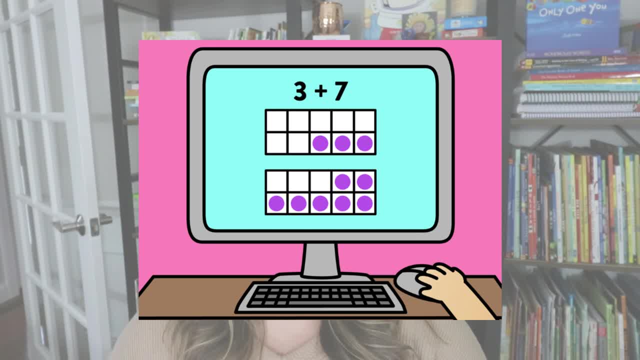 ones that my students already know. So by this point, if I am teaching them to make 10 in a larger- you know- addition problem, I want them to know those friendly pairs of 10.. And I also like the visual here so we can have students picture that we're taking those three dots and completing. 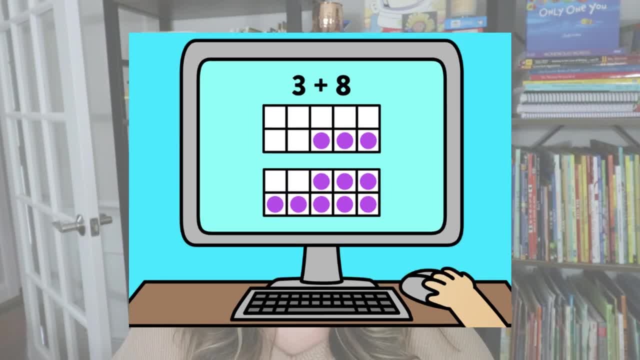 the 10 frame. So three plus seven. Then we go to the next slide. Okay, Well, if three plus seven was 10, what is three plus eight? And here we can see that it's 10 plus one more Again, I want. 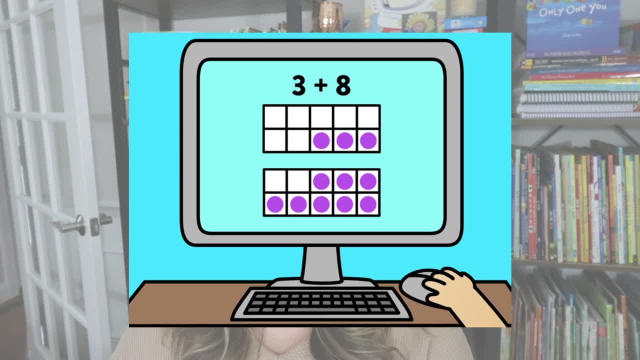 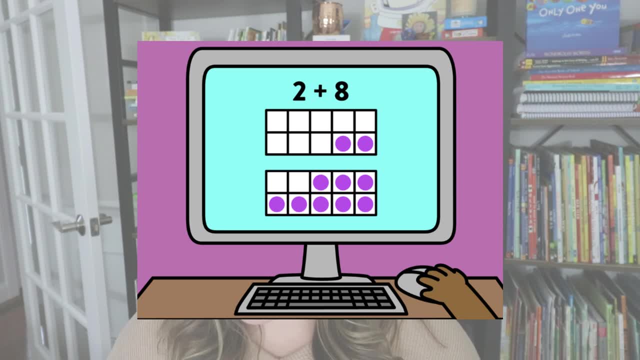 them to visualize completing that 10 frame by bringing two dots down and leaving one up. Then we go back to a helper problem: Two plus eight- We know that quickly makes 10.. So if two plus eight is 10, then two plus nine must be 11.. I'd probably do one more example like this: Four plus six. 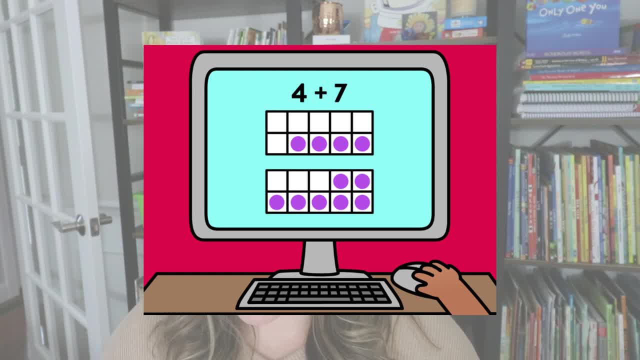 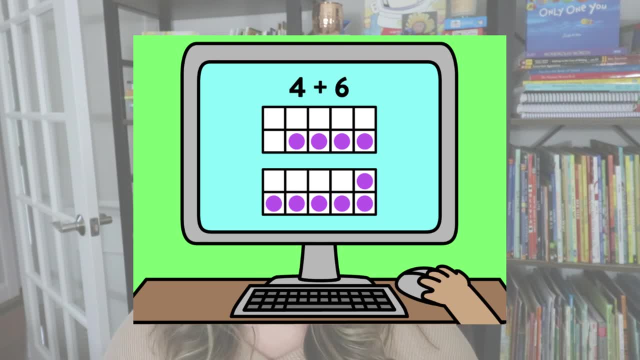 equals 10.. And then four plus seven must be one more, So it's 11.. And then I would go to something here. We'd go back to a base problem. Four plus six. Students might even say: hey, we just did that. 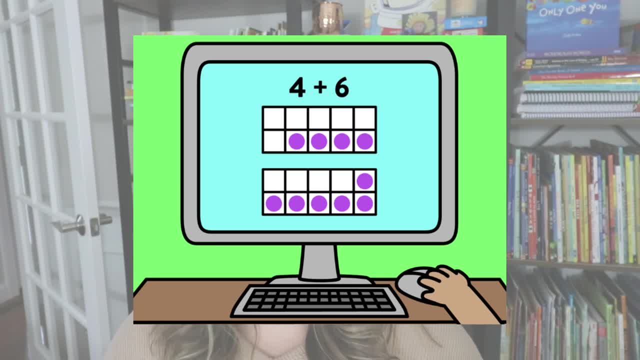 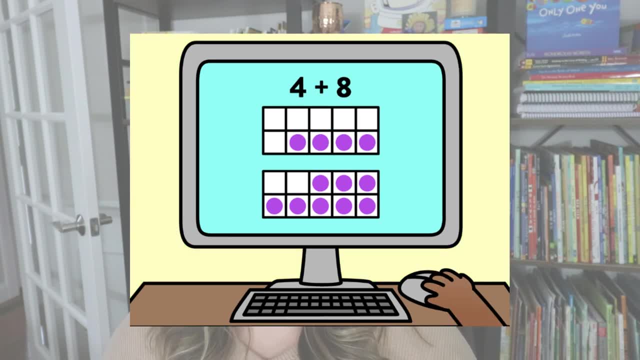 one. So we know four plus six is 10.. But now, instead of four plus seven, what's four plus eight? And here I'm having students fill in two of the dots there And then they have two left over. So four plus eight is 12.. So they're still making 10.. But instead of having one left over like they've been, 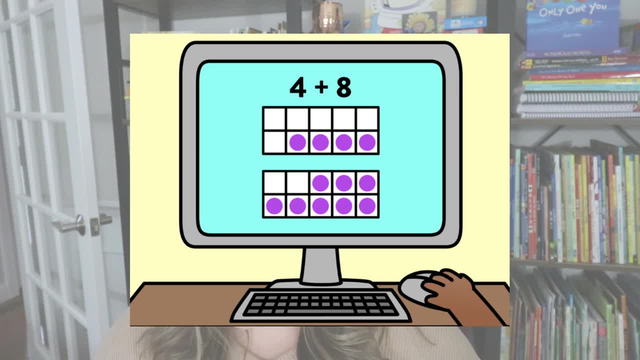 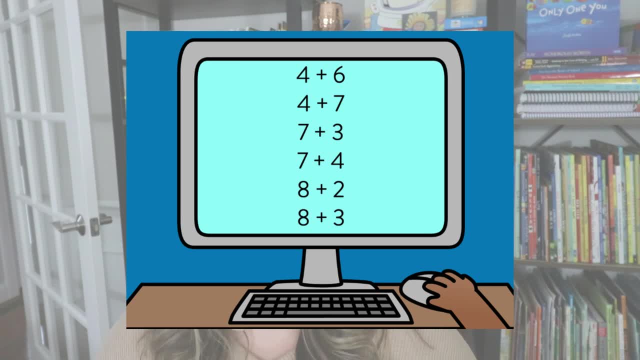 doing previously, they now have a few more left over. And then for some more abstract examples, when we have just our number sentences, we can use that as a reminder to always have those helper or base problems in there. So four plus six is 10, which means four plus seven is 11.. Go back to a helper, so on and so forth. I hope that allowed. 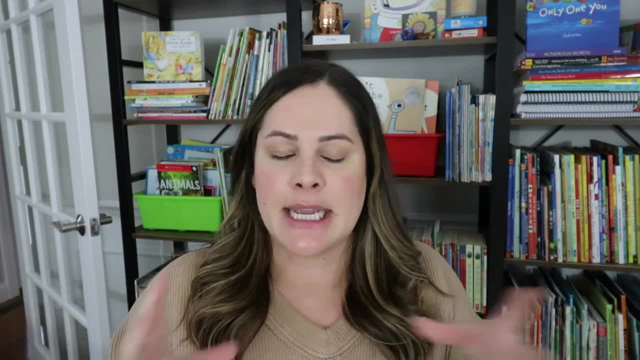 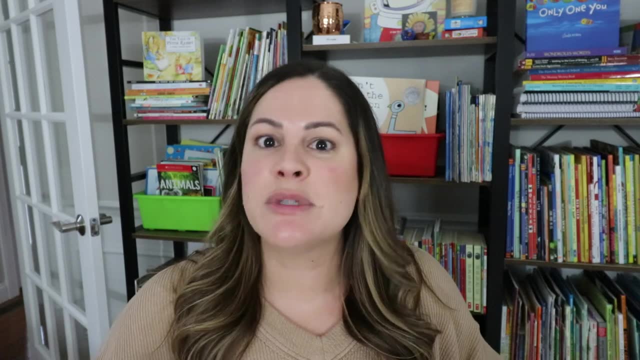 you to see that you can really use number strings or a set of related types of problems to teach many different addition and subtraction strategies that your students need to learn. By adding those visuals in there, it really helps students conceptualize the idea instead of just seeing. 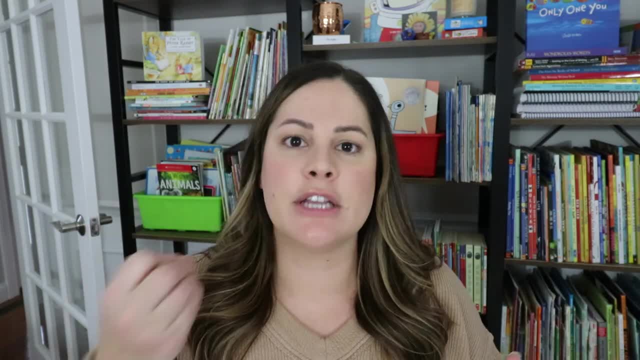 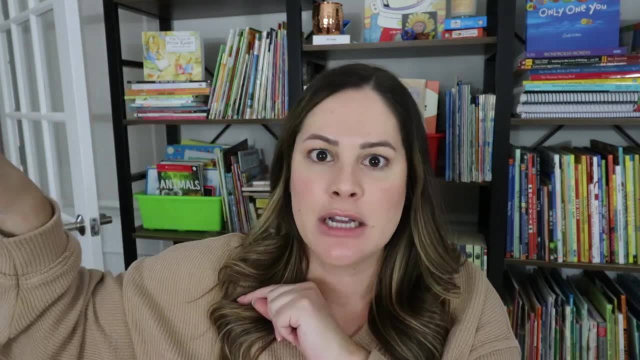 it in abstract ways. Now, the slides that I've been showing are ones that I actually already did, and I'm adding it to that bundle that I shared at the beginning with all the different types of math talks. So this one, of course, is going to be called number strings, And for each 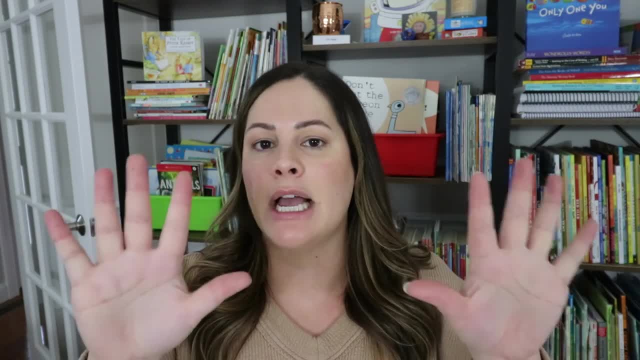 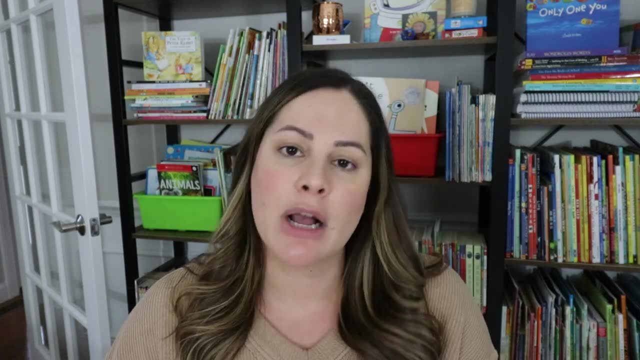 skill that we will work on. you will click on it and it will give you 10 slides. Now, in all of the math talks, there's always an editable slide if you want to add more or create your own of the same types of problems, And that will be true here as well. So I will give you some slides that match. 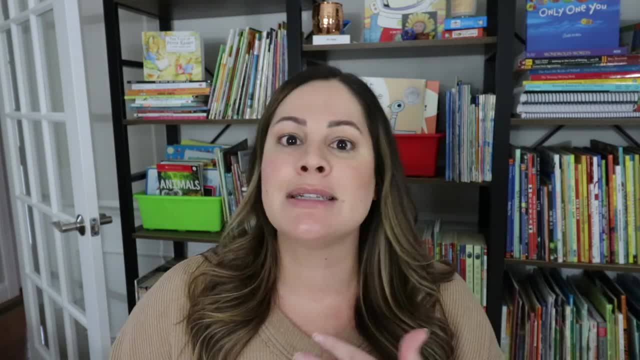 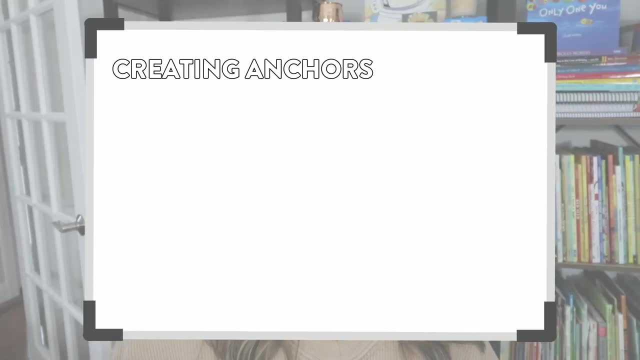 those that match the ones that your students have been working on, And if they need more practice, you can continue to create your own. Some of the strategies that will be included in this number strings unit include creating anchors of five and ten, making tens decomposing into friendly. 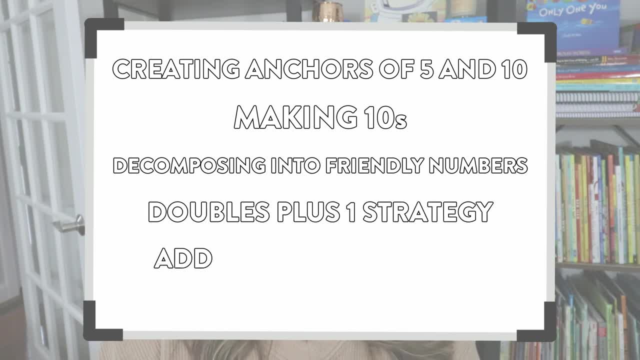 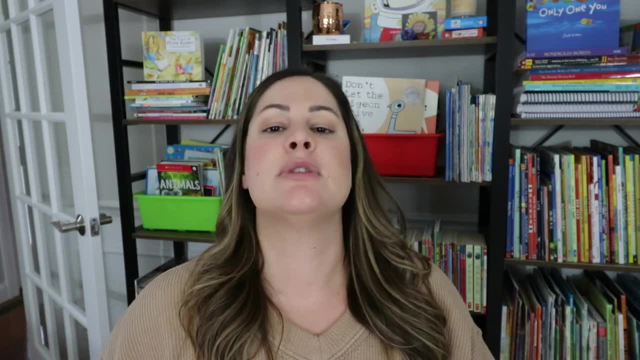 numbers, teaching doubles, plus one strategy adding multiples of ten and many more. Pretty much as I am brainstorming different strategies that I want to teach my students, especially going towards first and second grade. there's many more strategies they learn. I then try to compile.